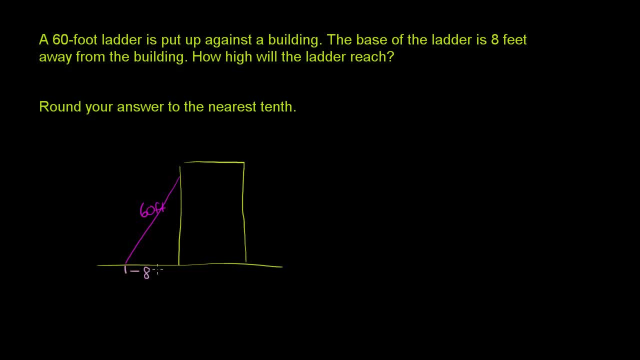 from the building. So this distance right over here is 8 feet And they say: how high will the ladder reach? So they want to figure out- or they want us to figure out- this height right over here. We need to figure out this height. 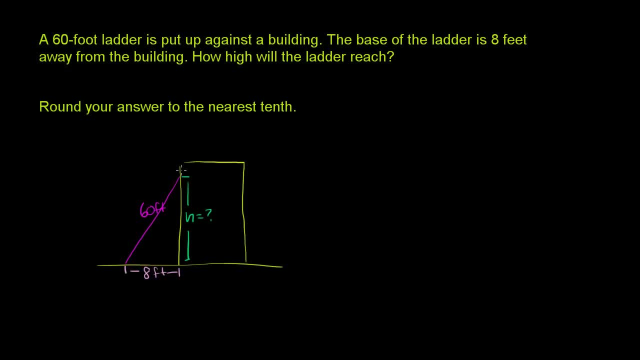 And, as we see, assuming that this is a normal building and it's built at a right angle to the ground, this triangle formed by the ladder, the building in the ground, is a right angle, It's a triangle, So the Pythagorean theorem will apply. 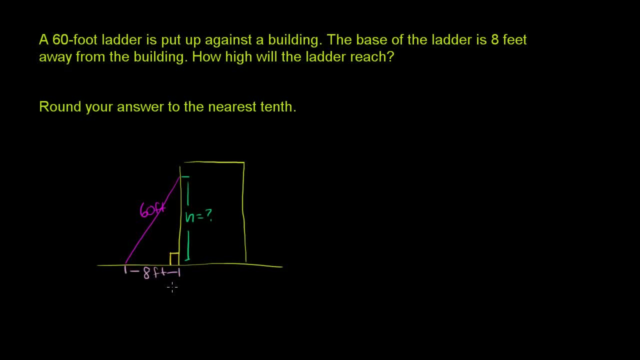 And the Pythagorean theorem tells us that the square, or the sum of the squares of the two shorter sides is going to be equal to the square of the longer side or the square of the hypotenuse, And the longest side is the side opposite the 90-degree angle. 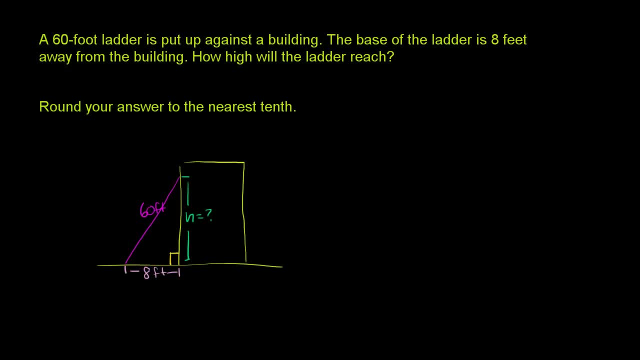 And that's the hypotenuse. So this tells us, the Pythagorean theorem tells us that 8 squared plus h, squared plus h, squared h for height, is going to be equal to 60 squared, And 8 squared is 64.. 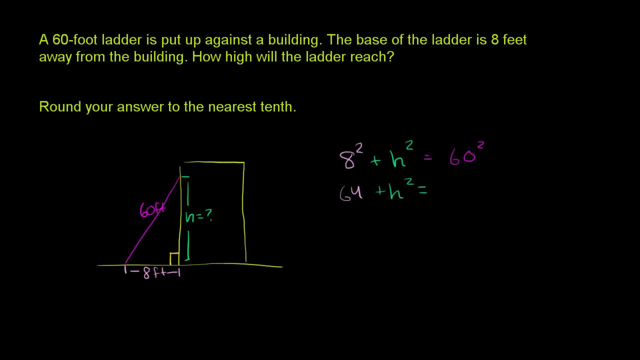 64 plus h squared is equal to 3,600.. Subtract 64 from both sides. So let's subtract 64 from both sides And we get h squared. h squared is going to be equal to what is this? 3,536.. 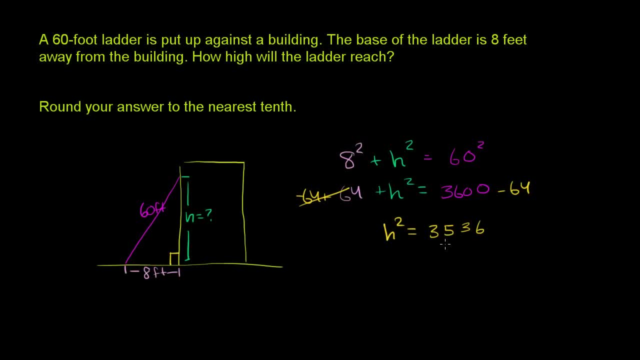 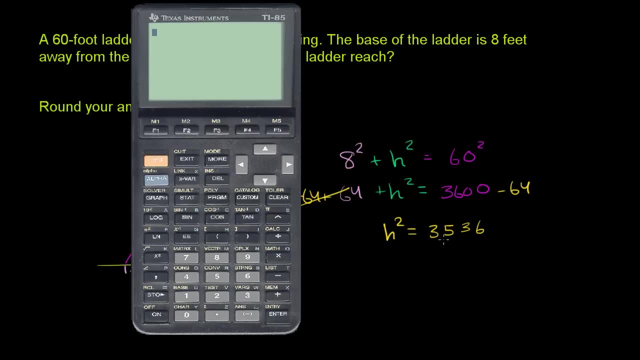 And then this doesn't pop out into my brain as some type of perfect square. So let's take a calculator out, So let's try it out. So we want to take the square root of 3,536.. So, second square root, you see a little square root symbol. 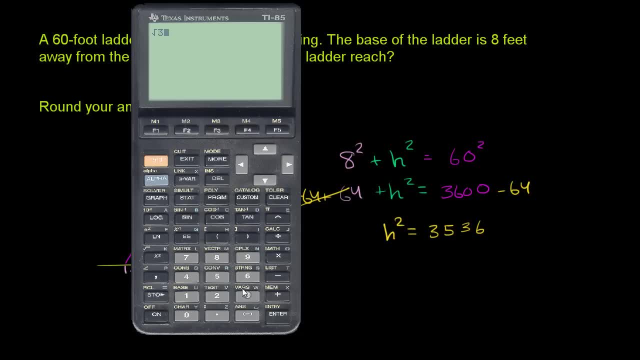 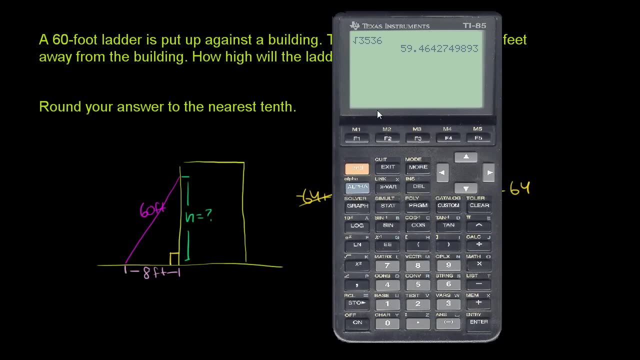 there in orange. That's why I had to press the orange button first. Square root of 3,536.. And I get 59.46.. And they want us to round. Let's round our answer to the nearest tenth, So 59.46.. 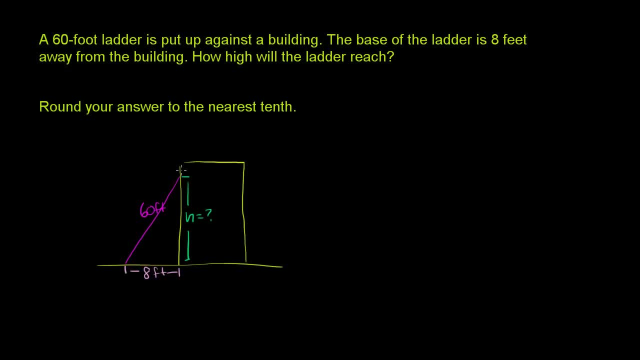 And, as we see, assuming that this is a normal building and it's built at a right angle to the ground, this triangle formed by the ladder, the building in the ground, is a right angle, It's a triangle, So the Pythagorean theorem will apply. 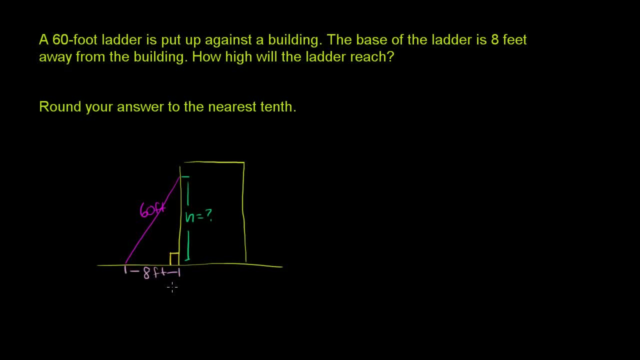 And the Pythagorean theorem tells us that the square, or the sum of the squares of the two shorter sides is going to be equal to the square of the longer side or the square of the hypotenuse, And the longest side is the side opposite the 90-degree angle. 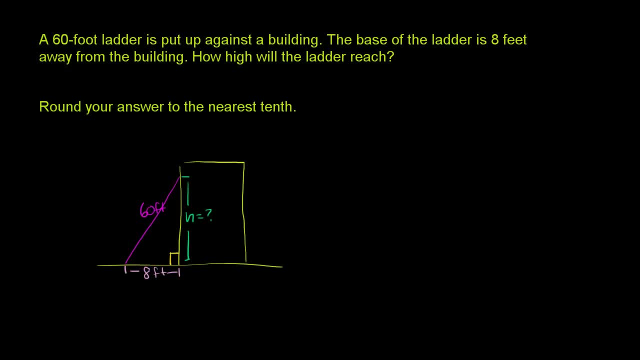 And that's the hypotenuse. So this tells us, the Pythagorean theorem tells us that 8 squared plus h, squared plus h, squared h for height, is going to be equal to 60 squared, And 8 squared is 64.. 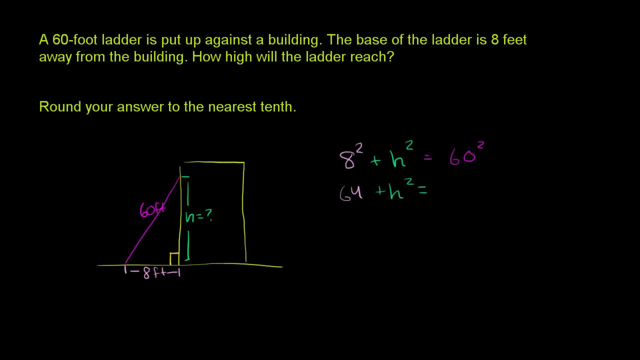 64 plus h squared is equal to 3,600.. Subtract 64 from both sides. So let's subtract 64 from both sides And we get h squared. h squared is going to be equal to what is this? 3,536.. 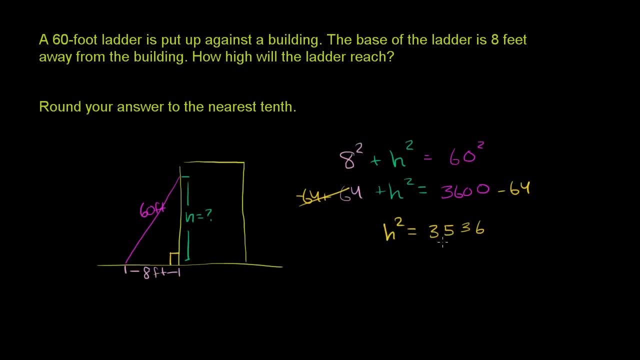 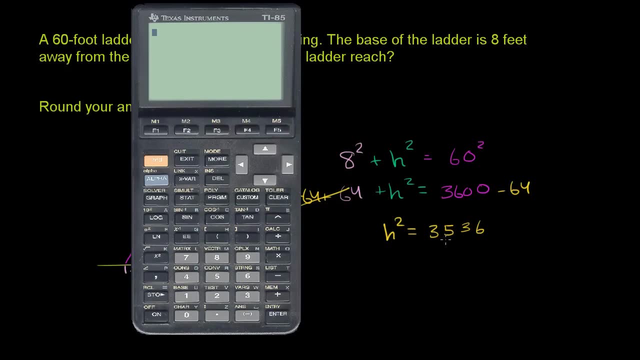 And then this doesn't pop out into my brain as some type of perfect square. So let's take a calculator out, So let's try it out. So we want to take the square root of 3,536.. So second square root, 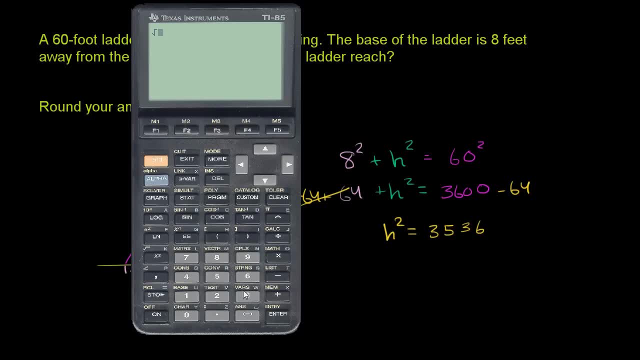 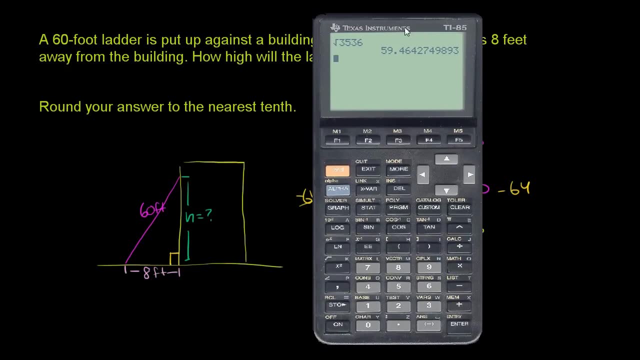 You see a little square root symbol there in orange. That's why I had to press the orange button first. Square root of 3,536.. And I get 59.46. And they want us to round. Let's round our answer to the nearest tenth. 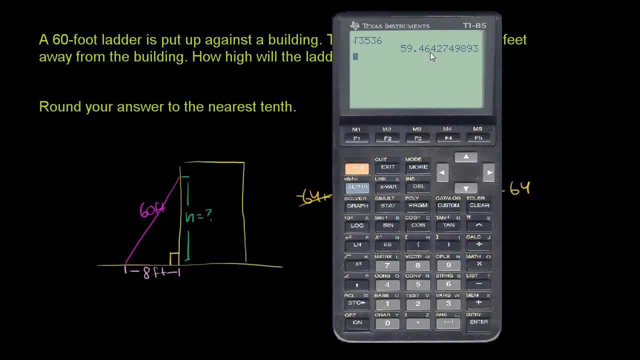 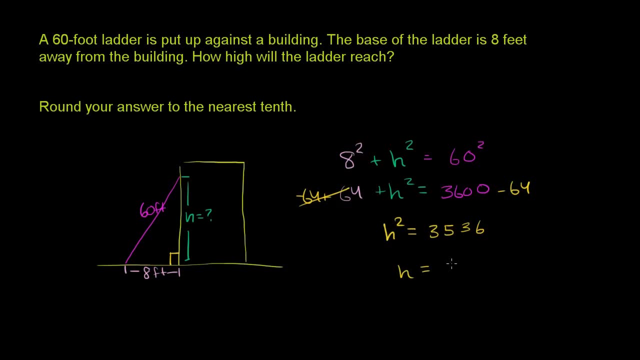 So 59.46.. 6 is greater than or equal to 5.. So round up, So it rounds up to 59.5.. So h is going to be equal to, maybe I should say approximately equal to- I already forgot the number 59.5.. 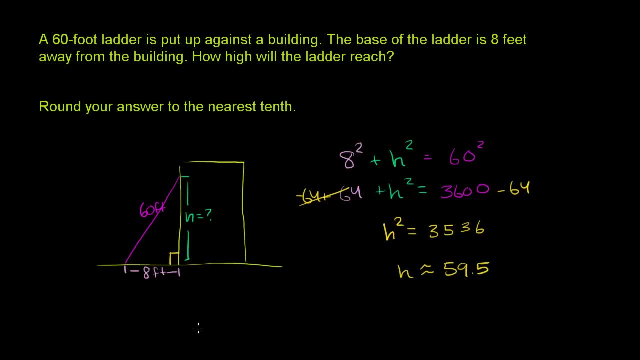 59.5. And we're done.